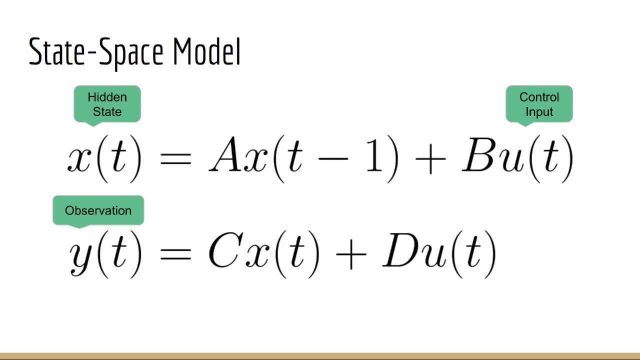 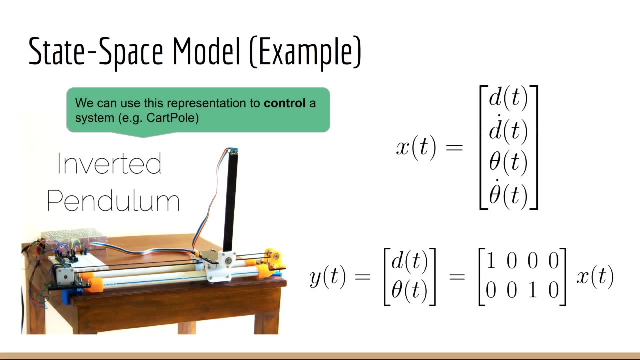 to our observation vector y of t. Sometimes y of t can also be directly affected by the control input u of t, but very often this is simply left out. In the second equation, by convention we call the matrices C and D. So just as a quick reminder of how such a state-space model might be used in the real 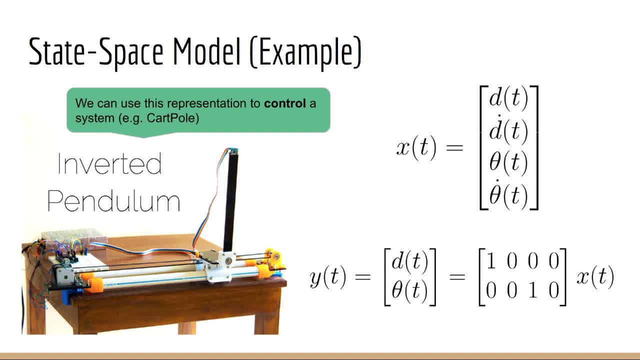 world recall that this is the set of equations that we use in control systems. An example of a real-world problem is the inverted pendulum, which you've seen if you've taken my courses on reinforcement learning. What's cool about typical courses on control systems is that 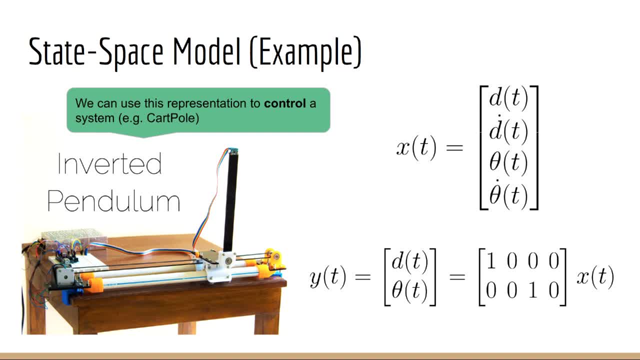 unlike reinforcement learning, we often get to work with real-world projects. So in the image here you can see an example of a live physical cart-pole system that can be controlled using the techniques of control theory. So as an example of how this relates to our equations, we might represent our state vector. 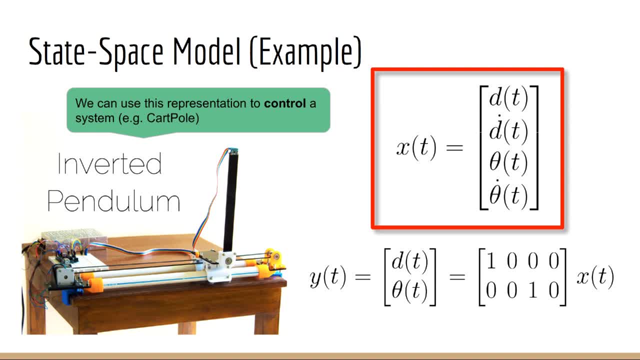 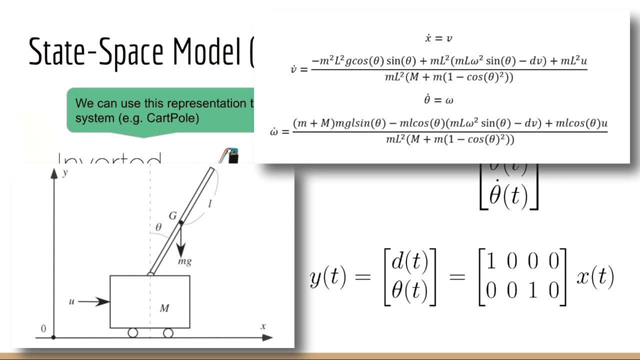 with four measurements, which are horizontal displacement, horizontal velocity, angle from the vertical and angular velocity, What we get to observe might only be the displacement and angle, since measuring velocity could be more difficult In practice. because this system is based on the laws of physics, we can use physics. 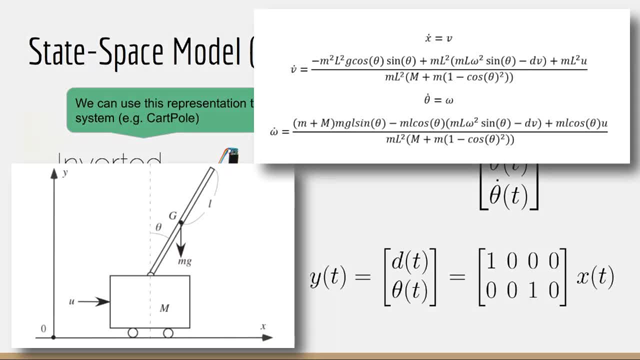 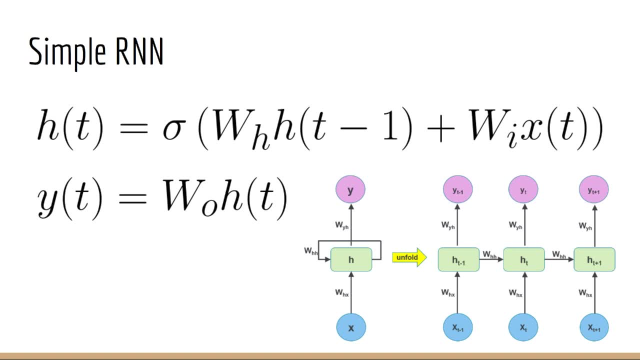 equations to determine the matrices A, B, C and D. Okay, so now let's recall the equations for a simple RNN. Suppose that we also include the output layer as well, and we assume that this RNN is many to many, meaning that we compute the output for every time step. 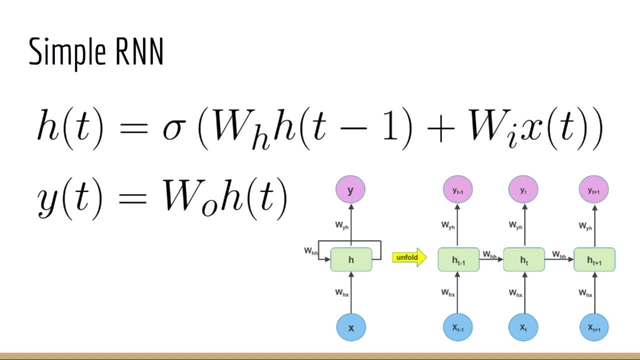 Note that, for simplicity, I've excluded bias terms. In this case, our hidden state vector is called H, which is dependent on the previous hidden state vector H and the model input X. They are related by the weights W and W with an activation function sigma. 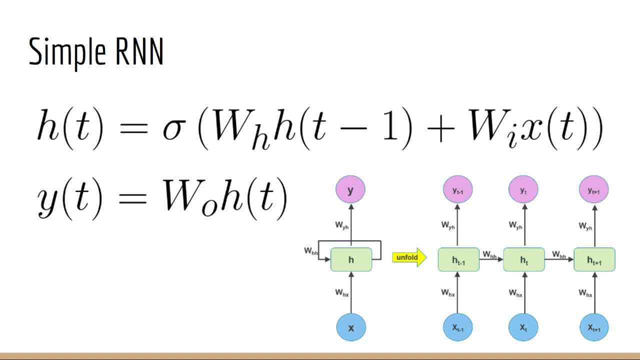 which can be the rel, u, tan, h and so forth. Furthermore, the output Y is related to the hidden state H using the weight matrix W output. Of course, at this point it should be obvious that the state-space model and the RNN are.